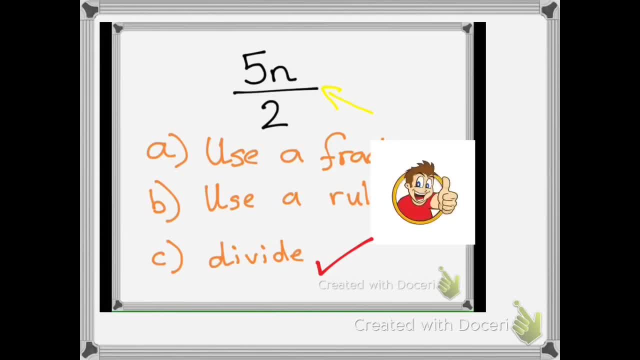 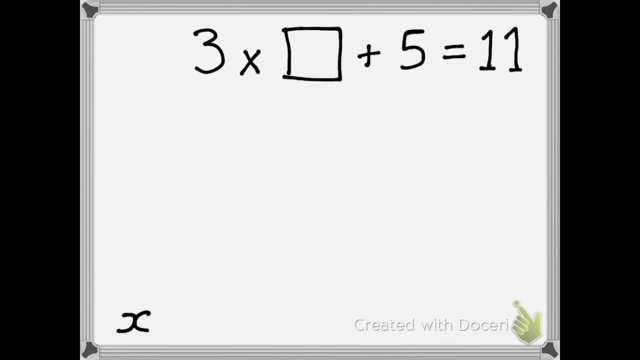 Give yourselves a big thumbs up if you got that one right. Okay, now moving on. Now, today, what we are going to be doing is we are going to be looking at questions and how we are going to express them algebraically. So basically, what that means is: 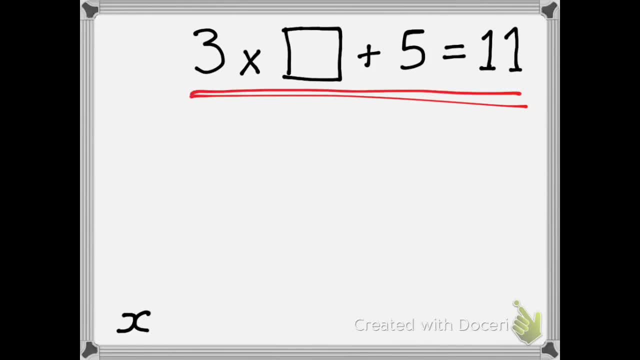 I'm going to turn this into an equation Now. the easiest way to do this is to start with the equals: what's on the other side of the equals? So I've got equals 12, so I'm just going to write that down there. Now, once I've written that there, I can scribble it out and I 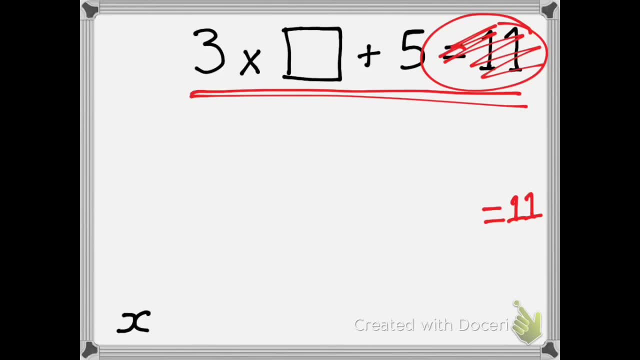 don't need to. I don't need to do anything with it now. Then I take a look at where there's a missing number. Now in algebra, what we do is, if there is a missing number, we can represent that by using a letter. So what I'm going to do 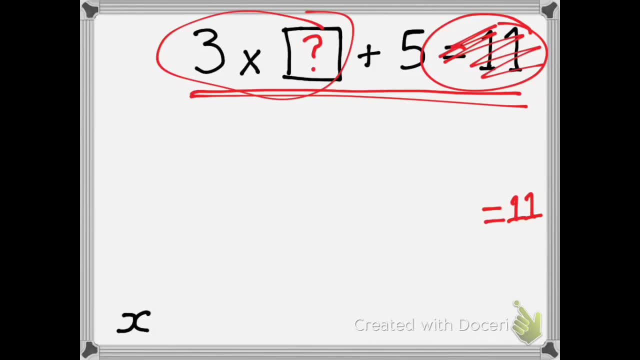 is. I'm just going to take a look at this little section here, because it says 3 multiplied by a missing number. Okay, so I can actually show that by doing 3x. Now, what you should know is that if there is a number next to a, 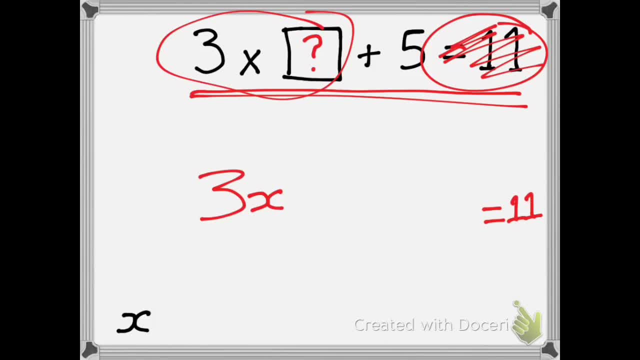 letter, then they multiply and that is the same as saying 3 multiplied by a mystery number. And what you might notice is that I've drawn the x a little, a little weird. and what we do is in algebra we draw our x's like this Because 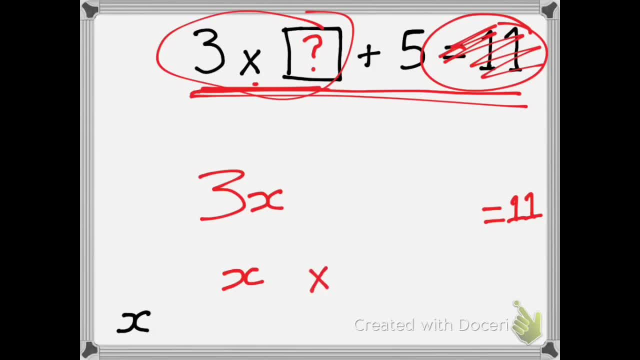 if I draw it like normal, like this, then some people might get confused between multiplication and x. Okay, so I've taken care of that bit now and I'm just left with plus 5, so I'm just going to keep that the same. So 3x plus 5 equals 11.. So I have taken that question to. 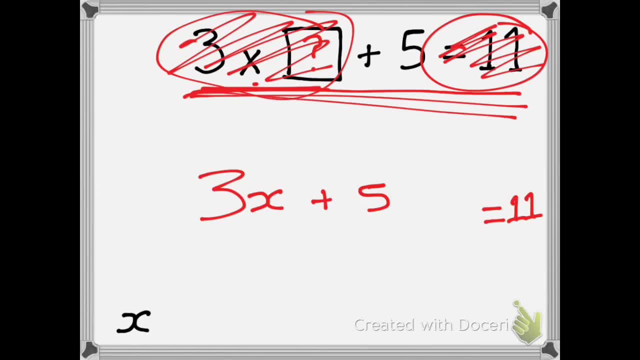 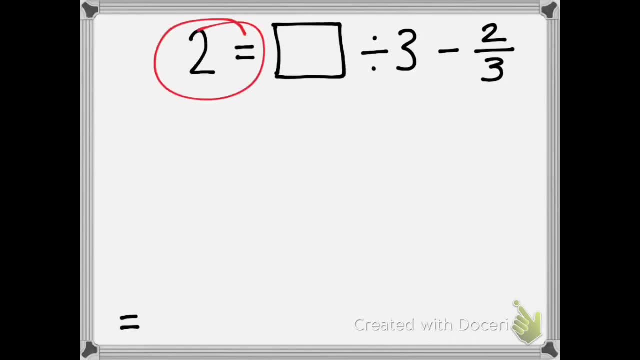 begin with, and I've expressed it now algebraically, I've expressed it with numbers Now moving on. Now, what you'll notice about this question is that the equals sign is actually before the question Now in algebra. you might see that quite often, and it's. please don't get confused about it, because it just means the same. 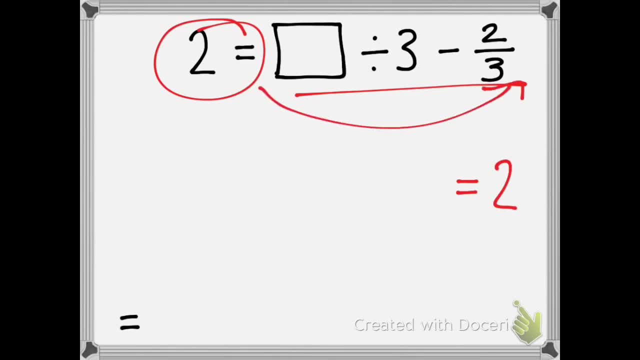 as if it was at the other side, at the end, like you're used to seeing it. Okay, it just means the same thing, Okay, so what I'm actually going to do is move it to the end of my expression here, my equation. So once I've done that, I can. 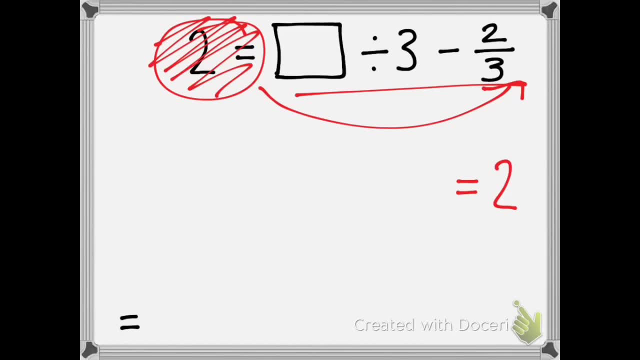 scribble that out, because I've finished with that. Now, this time I've got a divide. I've got a missing number divided by 3.. So instead of a missing number, I'm going to use x again and then divide by 3.. And if you remember what? 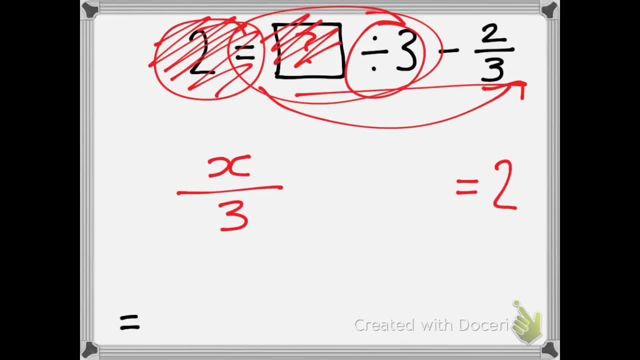 happened in the question right at the beginning of the video. you'll know that if I want to divide something and show it algebraically, I put a line and then a 3. So that means x divided by 3.. Okay, please don't write this. x divided by 3. 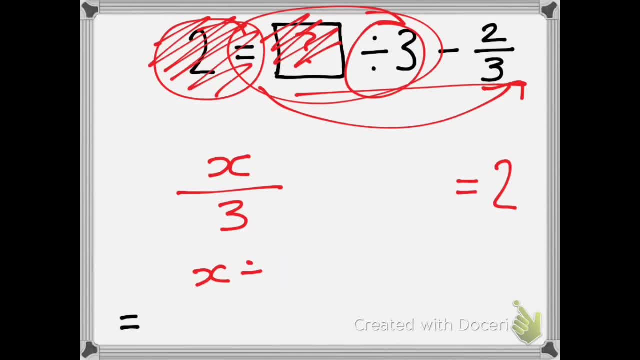 because we never see that in algebra. So now I've taken care of that part here. I'm just left with take away 2 thirds. There we go. So x over 3 or x divided by 3, take away 2 thirds gives me 2.. 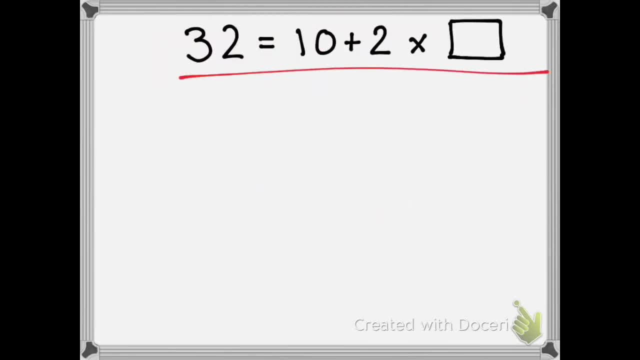 Now moving on to my next example. So again my question starts with 32 equals. Okay, so I'm going to move that to the back again: Equals 32.. So I've taken care of that part. Then I have. then I look for the missing number, So I've got 2 x. 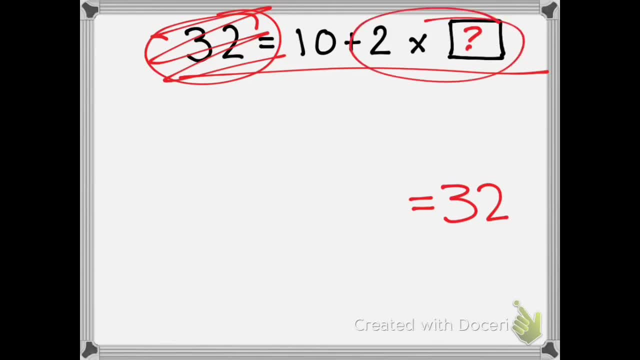 2 multiplied by a missing number. So again, I'm going to use x for my missing number, x, and then 2, and that would be 2 multiplied by whatever x is, And then I just add the 10.. Okay, now this question is a little bit different, because it's given to me as